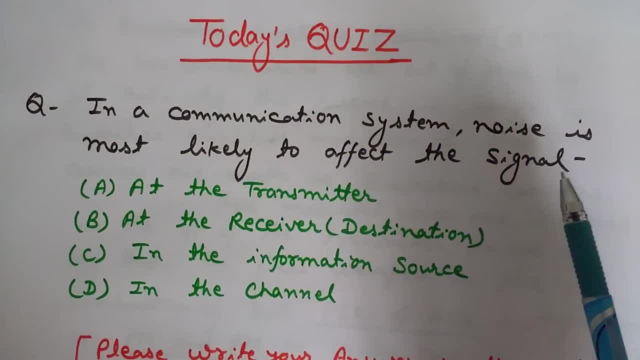 system, noise is most likely to affect the signal. At which stage? At the transmitter? second option is at the receiving or the destination end, in the information source or in the channel. So if you know the answer of this question, please write your answer in the. 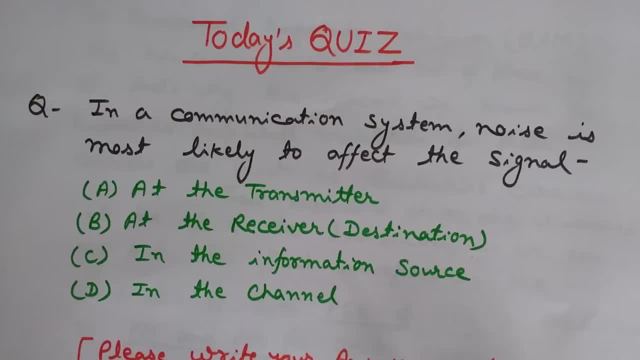 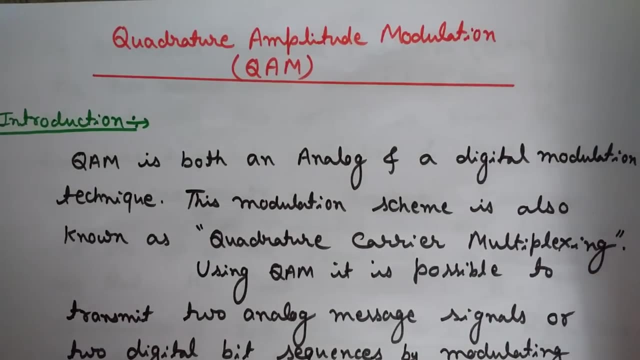 comments, and we will ask such simple questions in every video lecture and you will have to write your answer in the comments. So now let's come back to our topic: Quadrature Amplitude Modulation, the basic concept. We can use this Quadrature Amplitude Modulation with either 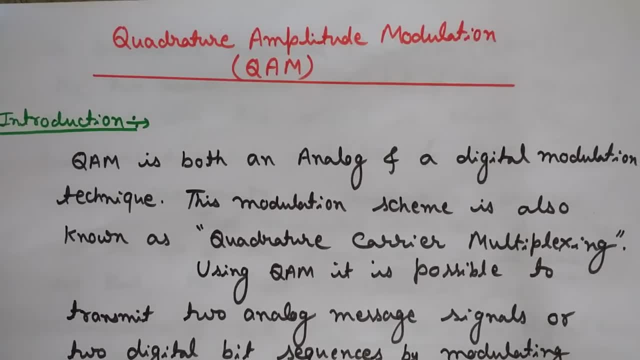 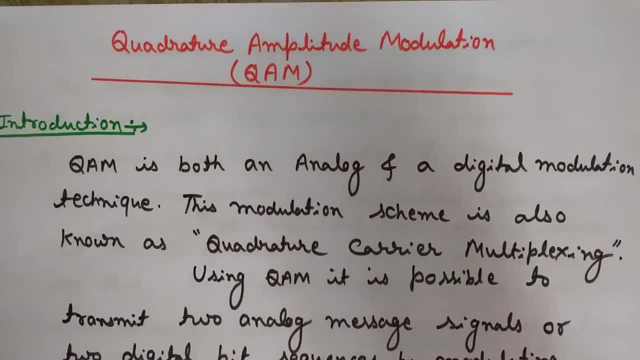 two signals. If we use it with analog messages, then we have two analog message signals and they are amplitude modulator and we have two carrier waves. So in QAM technique, if we use it with analog modulation, then we use amplitude modulation and with the digital, 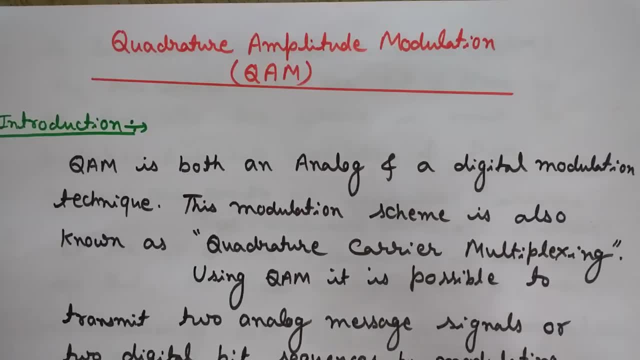 bit streams. if the message signal is in the form of digital bit streams or digital bit sequences, then we use ASK modulation, that is, Amplitude Shift Keying Modulation. So why this is known as Quadrature Amplitude Modulation? What is the meaning of Quadrature? 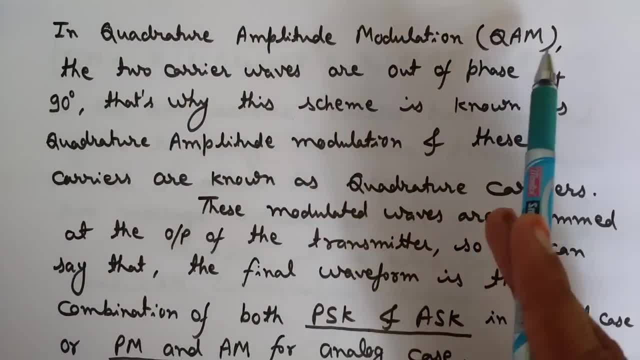 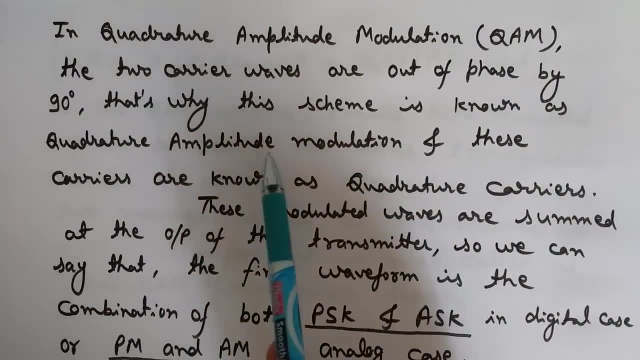 here. Actually, in Quadrature Amplitude Modulation, QAM, the two carrier waves are out of phase by 90 degrees. That's why this scheme is known as Quadrature Amplitude Modulation And these carriers are known as Quadrature Carriers. Let me show you this with the help of a block. 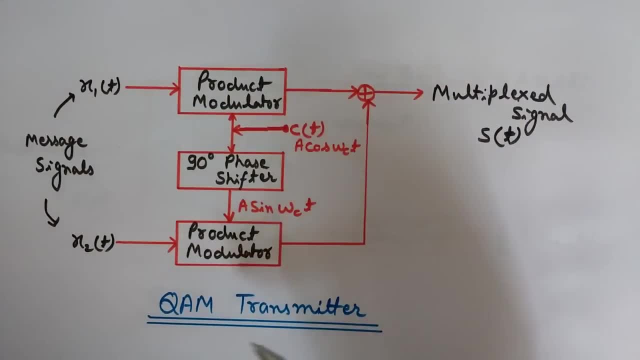 diagram. Look at this block diagram of the Quadrature Amplitude Modulation transmitter. Here we have two message signals: X1T and X2T. x to t. these are the. this is the case of analog. okay, these are the analog messages and we are. 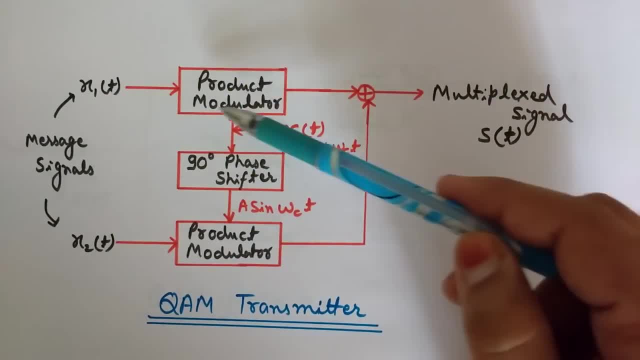 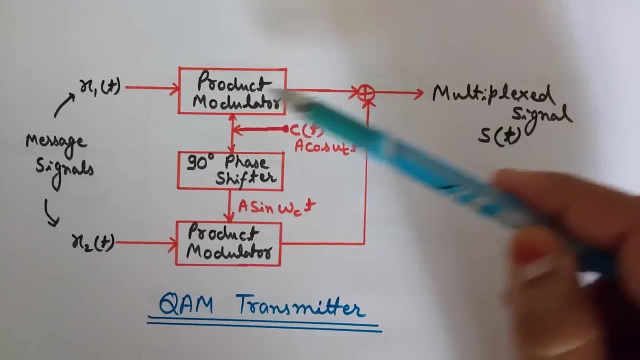 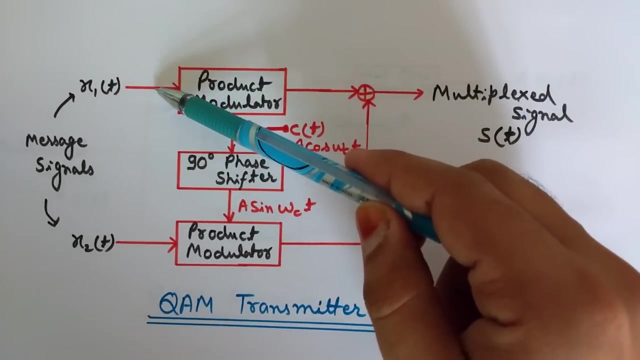 using the product modulators, two product modulators, modulators. you see here that the output here is nothing but the amplitude modulated wave, because here we are using this. this product modulators inputs are message signal, analog message, modulating signal, and here we are supplying the carrier wave. 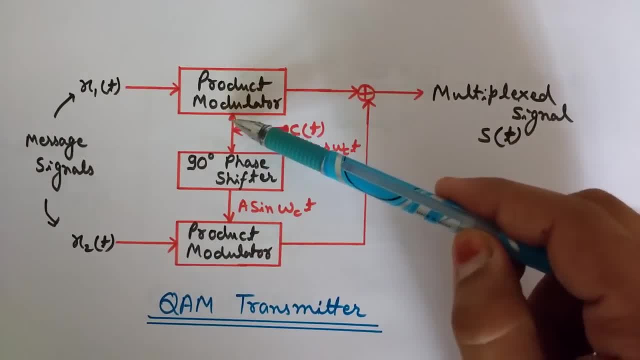 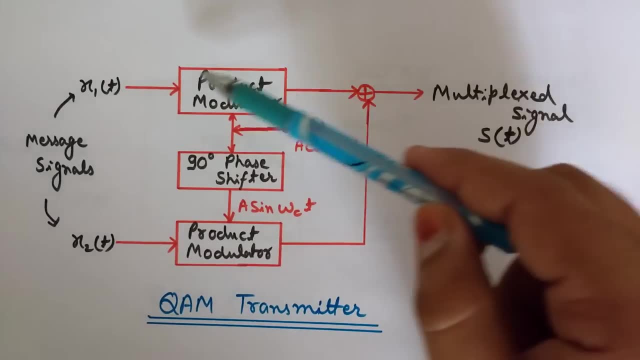 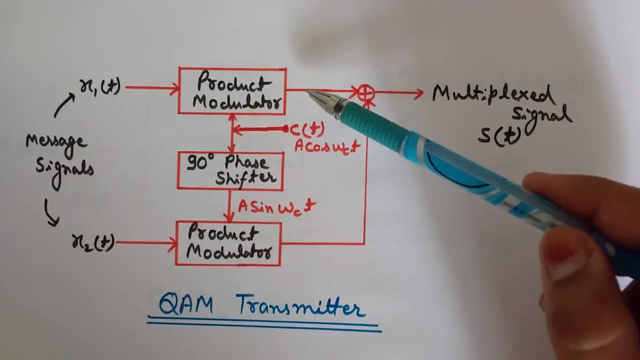 a, cos, omega, ct. this is the carrier wave and these are the two inputs for this product modulator and in the output we will get am amplitude modulated wave. because when modulating signal and carrier waves are applied to the product modulator, then the output gives us the double sideband suppressed. 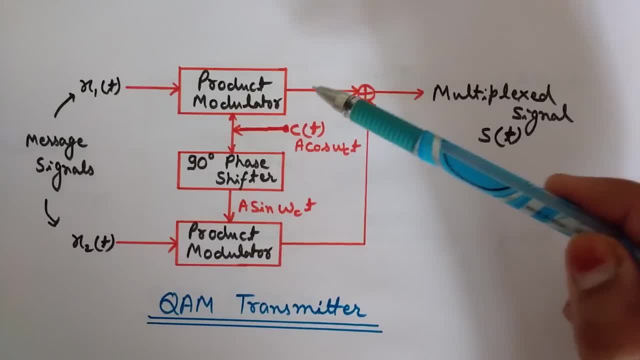 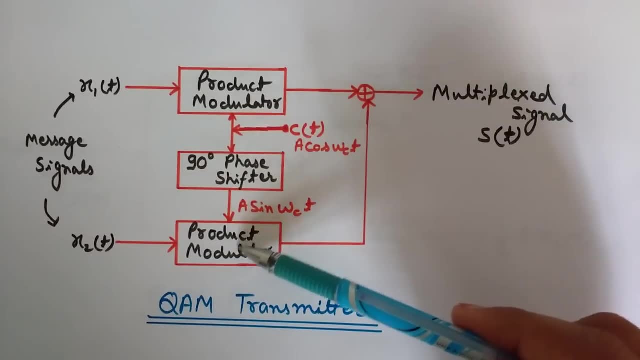 carrier dsbsc, double sideband suppressed carrier output, which is a form of amplitude modulation. and here also look at this- this product modulators, two inputs are having the carrier wave and the modulating signal. but here the difference is that here the carrier wave is first applied here and then it is phase shifted by 90 degrees, so 90 degree phase. 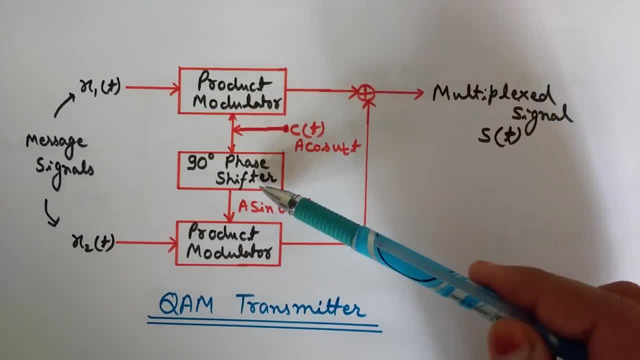 shift. shift takes place in this 90 degree phase shifter and then the output is a sine omega, ct. when we phase shift the cos wave by 90 degree, then then we get the sine wave. so its inputs are the modulating signal, another modulating signal, x to t. 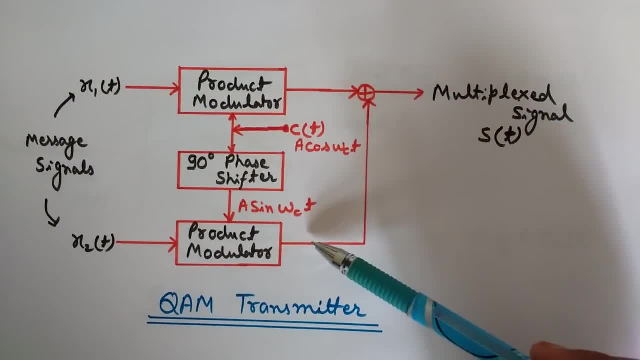 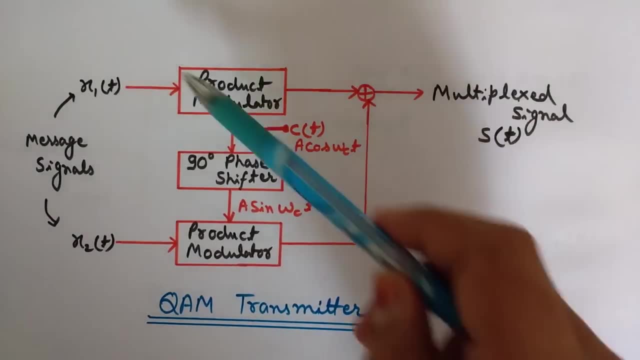 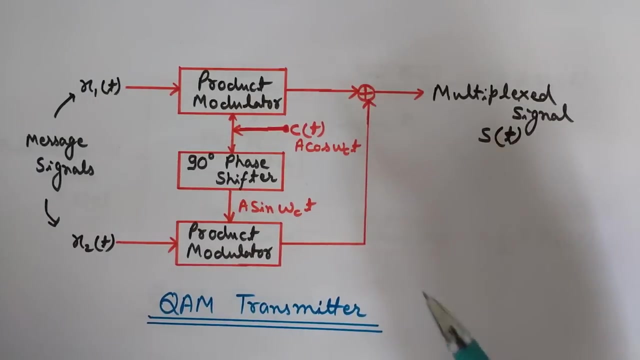 phase shifted carrier wave, so the output is again the amplitude modulated wave. now here you can see that this is a combination of- if we talk about analog kind of modulation, then this q a m quadrature amplitude modulation is a combination of both amplitude modulation and the phase modulation. 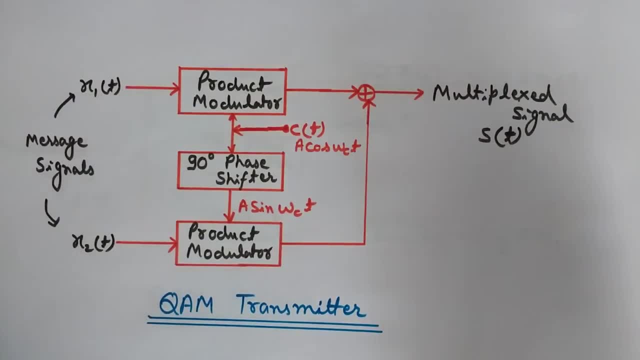 because phase shift is also there. so if this is the case for amplitude, this is the case for analog modulation. now, in case of digital, if you talk about digital, then at this place there will a stream of a digital bits, okay, and we will have a combination of phase shift keying. 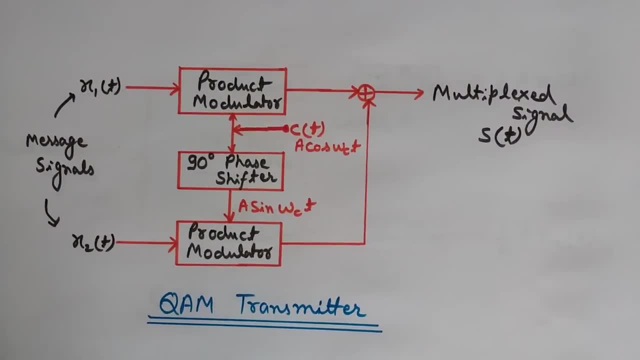 p s k and a s k, amplitude shift keying of both of these. so in digital case q a m is a combination of a s k and p s k. okay, and at the output these outputs are taken of the these am modulator waves are taken and the output here we get is multiplexed signal. so this is known. 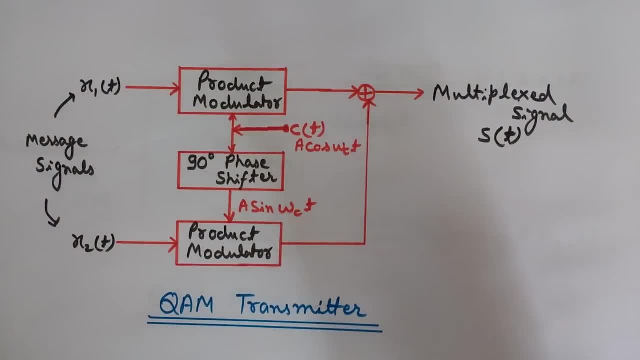 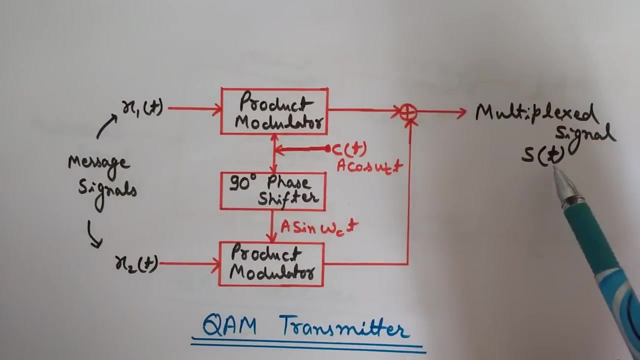 as quadrature amplitude modulation because we phase shift the carrier wave by 90 degrees. this is the reason, okay, why it is called as quadrature. so in this q a m transmitters block diagram, you can understand that the output s? t would be this: okay, this s? t would be x 1 t. 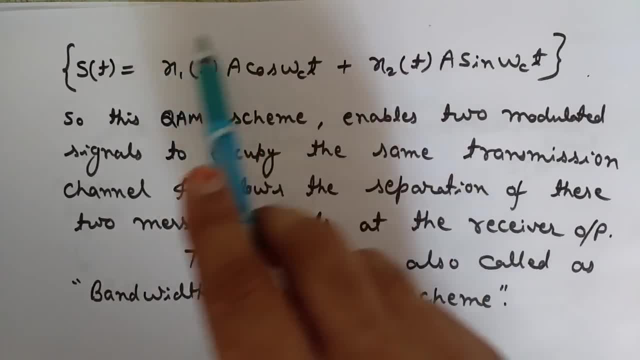 a, cos, omega, c, t, the output of the product modulator. first product modulator that it will, it will provide the product of these two terms, this carrier wave and the first modulating signal: x, 1, t. and this is the second modulating signal and the carrier. 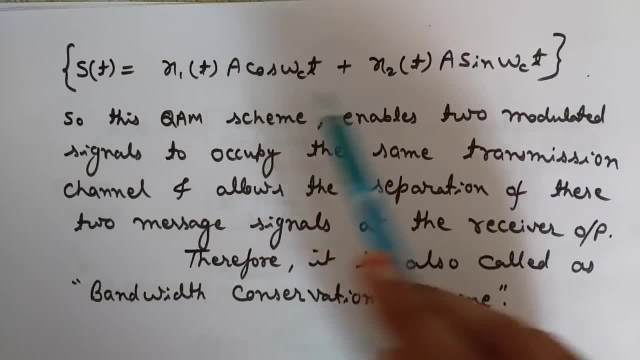 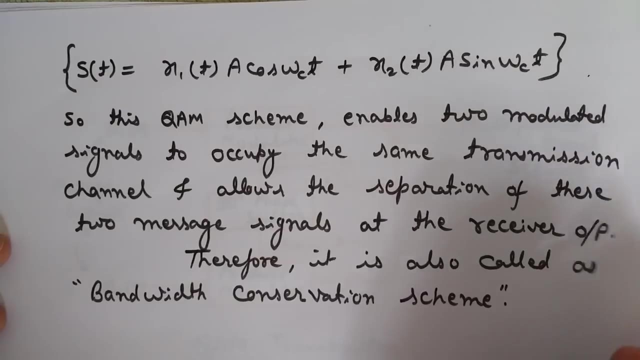 wave with a phase shift of 90 degrees. that is cos changed to sine. okay, so x 2 t, a sine, omega c, t and, as we know that they have been added in the output, so this is the s? t. if you want to see the diagram, let me show it to you again. the output of this product modulator is: 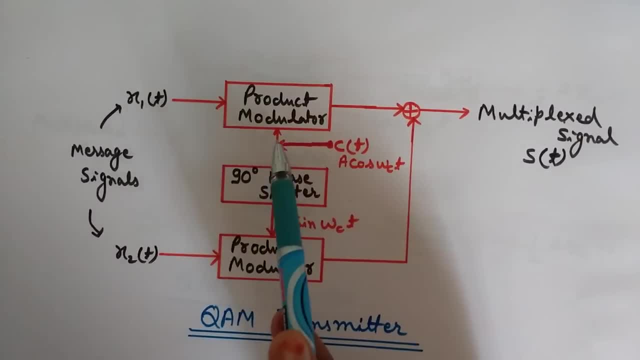 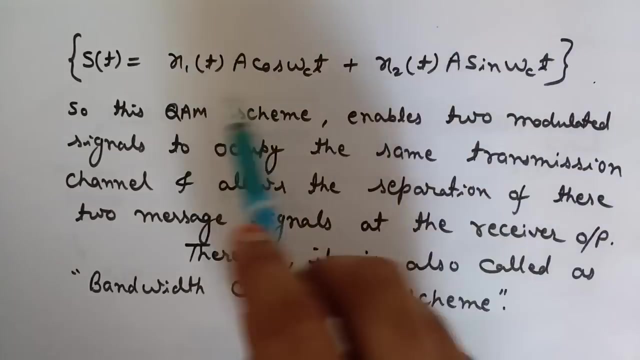 x 1 t a cos omega c t, multiplication of this and this, and output of this one is the multiplication of this and this. so it is x 2 t a sine omega c t, and we have added them. so we add these two terms and this is the s? t combined expression. okay, so one important thing. you should also know that this 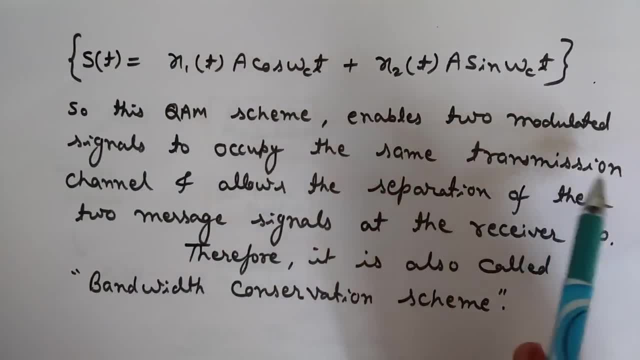 q a m scheme enables two modulated signals to occupy the same transmission channel and allows the separation of these two message signals at the receiver output. therefore, it is also called as bandwidth conservation scheme because with with this scheme, what we are doing? we are simultaneously transmitting two analog signals. 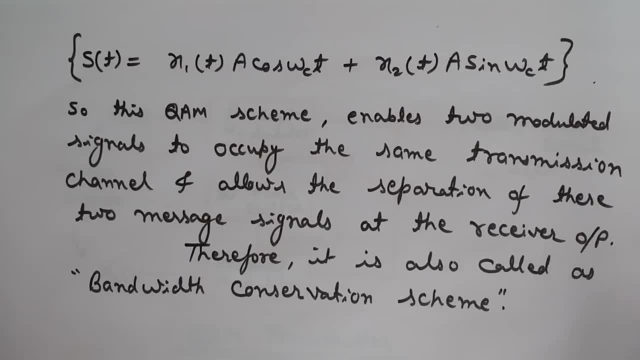 and are in line with the product modulator distribution. once these two, present to the messenger, confess to the product modulator, we are transferring these two message signals to the product modulator, and the two modulator waves are using some of these. så in doing this we are simply sending two significa signals to the carrier at those two wave numbers. 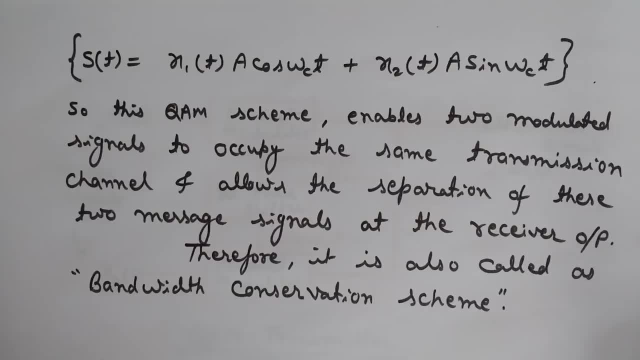 that are capable of our system自. I have a dw size of 99 degrees so we are doing the sampling Canadians. so I will show you how I am showing you how our system is targeting these wave counters. to my інthe section forty five, Lars pro g? dem is providing two Signal message: signals to the product model. 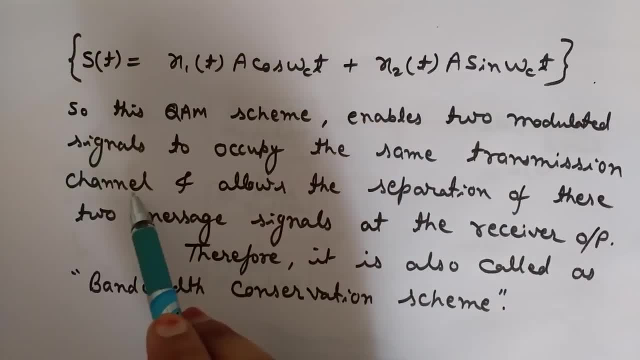 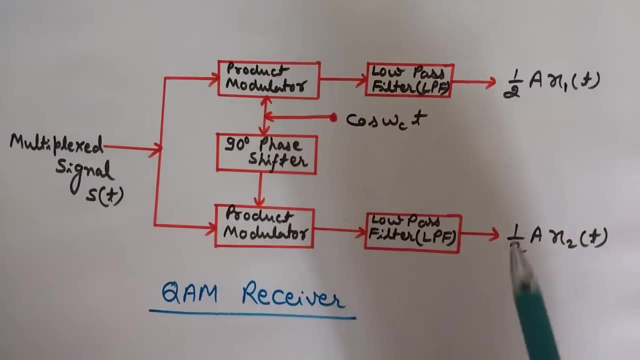 scheme allows us to occupy the same transmission channel and at the receiving end we can detect these message signals easily. therefore, we call this scheme as bandwidth conservation scheme also. so this is very important scheme. now let's have a look at the block diagram of a qam receiver. this: 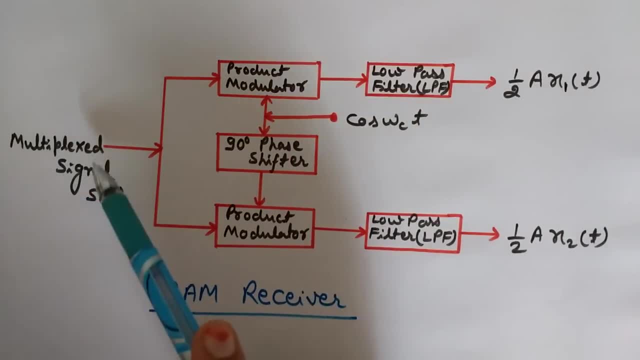 is the qam receivers block diagram and here the multiplexed signal st. this was the output of the qam transmitter. this is the multiplex signal st that we have seen the equation of st, so this has been applied. this is the input to this qam receiver and this has been applied to this. 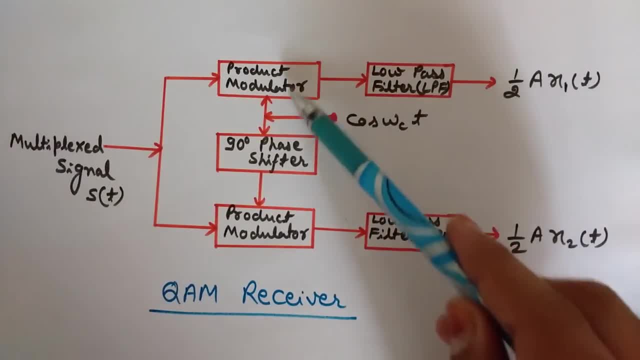 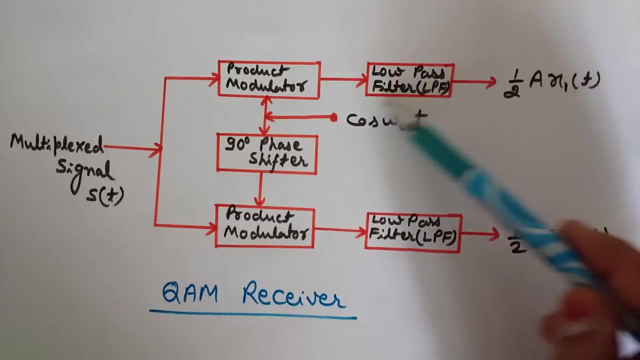 receiver. and now again, we use two product modulators and 90 degree phase shifter and apply this st signal again to this product modulator, to both of these product product modulators and this phase shifter. again this, this cos omega ct, is applied to this qam receiver and this qam transmitter is applied to this qam receiver. 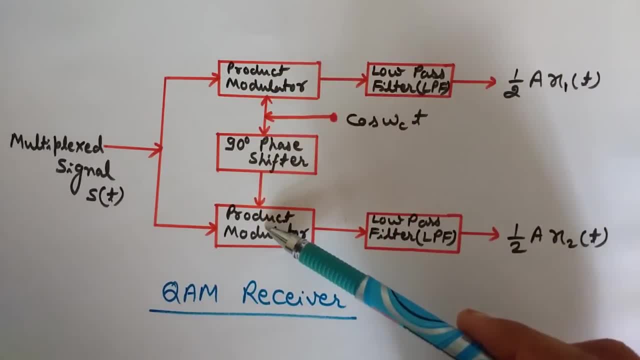 directly to this product modulator, while to this product modulator we have first input, as this st output of the transmitter multiplex signal and this carrier wave is phase shifted first by 90 degrees and then applied to this, and after passing them through the low pass filter, we get at the 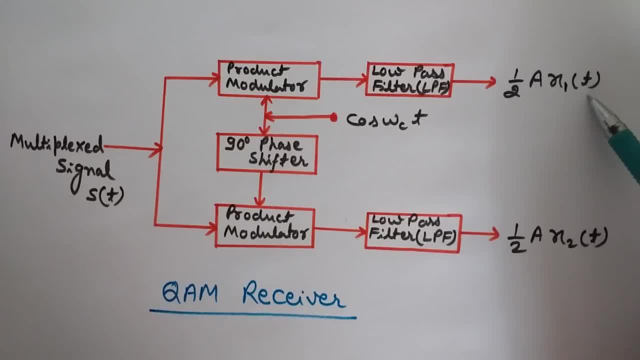 output our modulating signal: x1t at this output and x2t at its, at the output of this low pass filter. but important thing here that should be taken care of is that this cos, omega ct, this carrier wave, this oscillator and the oscillator used at the transmitting end, okay at this place. 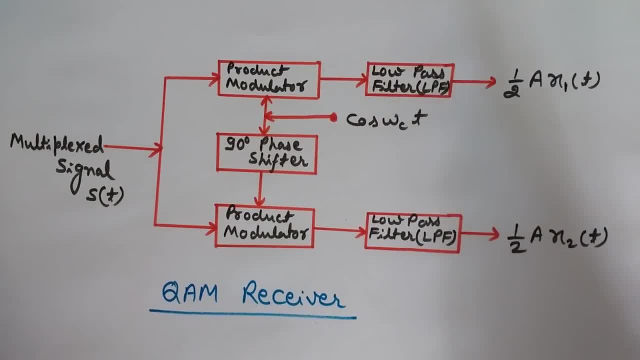 should be in coherence. they should be in same phase. okay, so this is the condition: carrier wave used at the transmitter and at the receiving end. they should be in phase, okay. so in this way we again get the modulating signals back at the receiving end. this so i think you understood all the points. 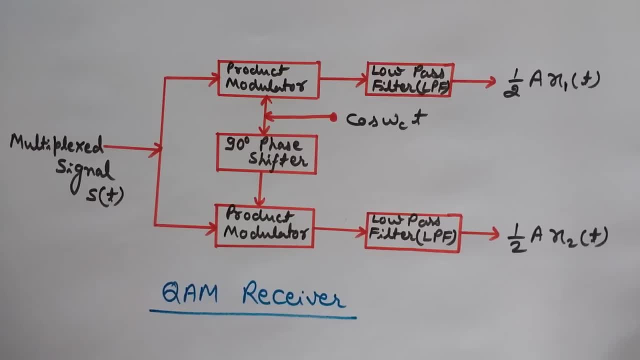 in the next videos we will see another modulation techniques. if you like my video, please click on the like button and if you have not subscribed my channel yet, please subscribe my channel. engineering made easy. and yes, don't forget to answer the question that i have asked you. 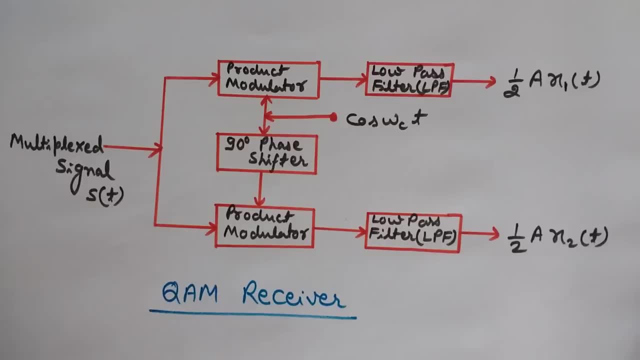 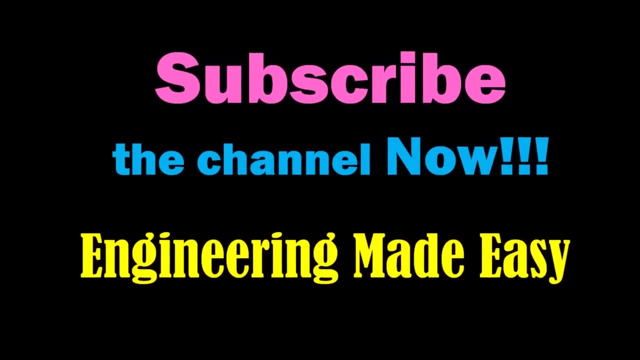 in the starting of this video. write your answer in the comment section of this video. till then, bye, bye. see you soon in the next video. thanks for watching friends. for more such videos you can subscribe my channel- engineering made easy. and please don't forget to like and share the video.